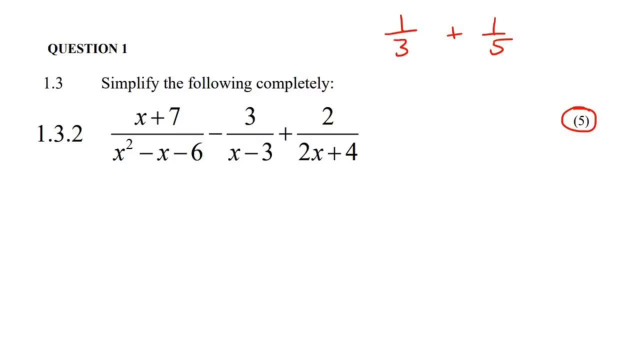 what would you do- Well, well done- if you said you would get a common denominator. Whenever you plus and minus fractions, you need to get a common denominator. So that's an important step. We need to get a lowest common denominator, But to get your denominators you have to make sure. 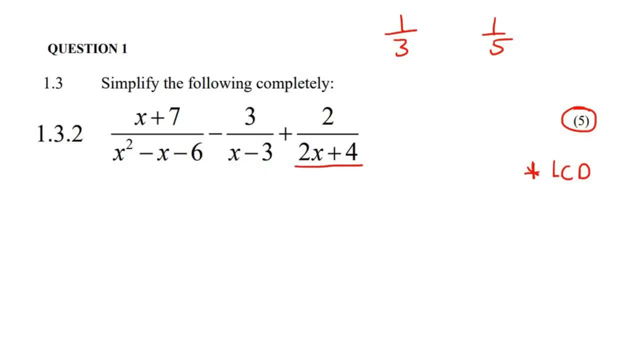 that they are all factorized. Okay, So this one can be factorized and this is a trinomial, So that can be factorized. So that'll be our first step. Let's just go factorize, Because if we don't, then you're going to tell me: oh, these two parts are completely different, but maybe they. 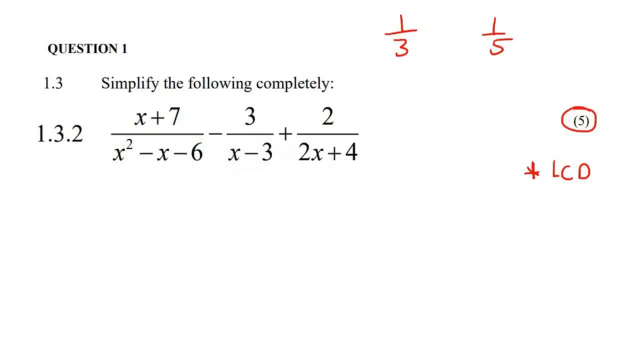 not. If you factorize this, maybe it ends up looking very similar to that. Okay, So X plus seven. Now, if you factorize, this is a trinomial, So let's factorize that over here together. So we look at the number six Now. 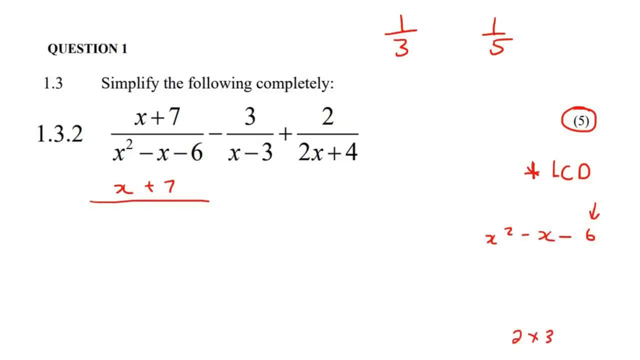 we know that the number six can be written as two times three or one times six. Now, which one should we choose? Should we choose the one in the six, or should we choose the two in the three? Well, how do we work this out? What we do is we look at this term here in the middle, with 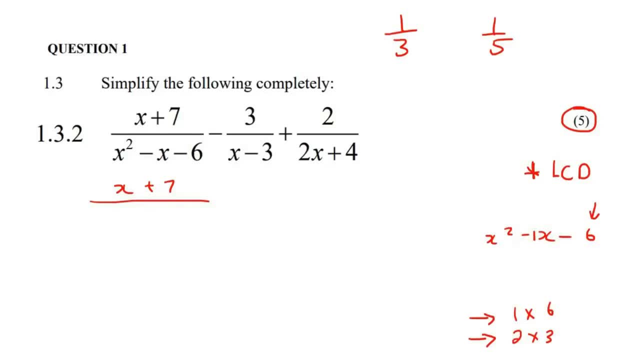 the X And we try to make minus one. So you cannot make minus one using these two numbers, Like six minus one is five. One minus six is negative five. One plus six is seven. You're not going to be able to do it, So it's not that one, So we're going to use these two. How do you make minus one? Well, 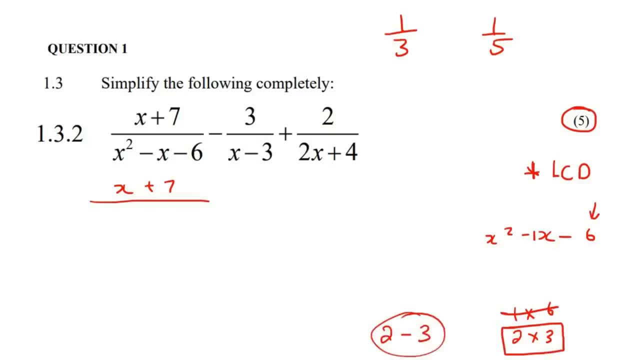 you say two minus three, because that gives you minus one. So we're going to open up two brackets, Okay, And we're going to say X and X, And then we're going to say positive two for this one because it's positive. And then we're going to say positive two for this one because it's positive. 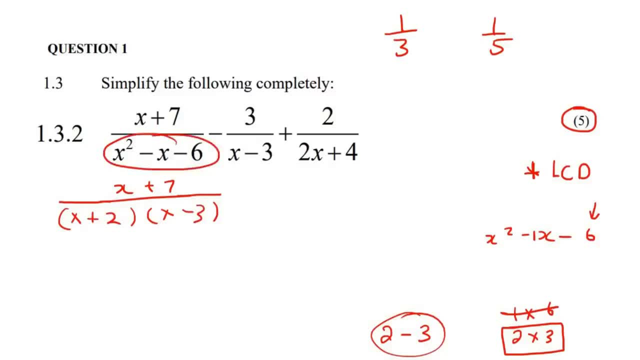 And then negative three, And that is how you factorize that part. Okay, Look at that. X minus three, X minus three- Ooh, something similar. Okay, Now we're just going to leave this part, because this is already factorized. Okay, Now, here you can take out a common factor. 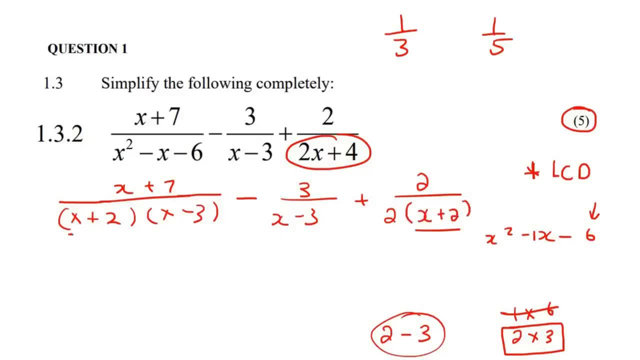 A lot of learners forget about that. And look at that X plus two, X plus two hashtag just saying So you guys must look out for that. Okay, Now to find your lowest common denominator. all you do is you just take all the different parts. 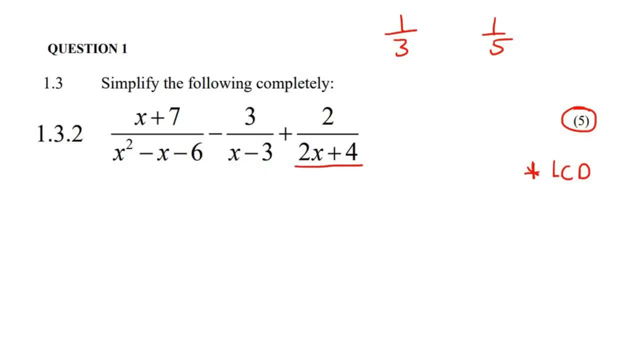 that they are all factorized. Okay, So this one can be factorized and this is a trinomial, So that can be factorized. So that'll be our first step. Let's just go factorize, Because if we don't, then you're going to tell me: oh, these two parts are completely different, but maybe they. 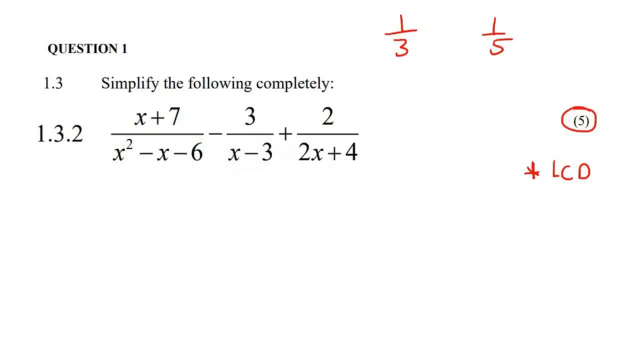 not. If you factorize this, maybe it ends up looking very similar to that. Okay, So X plus seven. Now, if you factorize, this is a trinomial, So let's factorize that over here together. So we look at the number six Now. 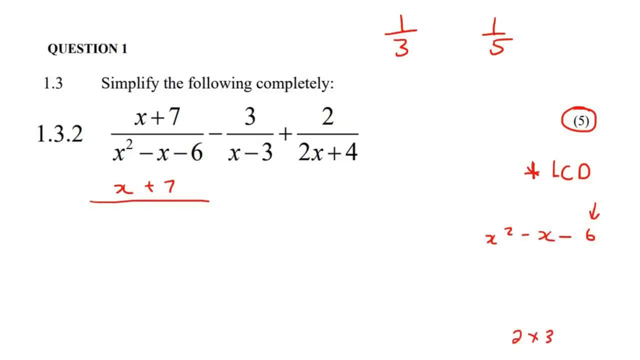 we know that the number six can be written as two times three or one times six. Now, which one should we choose? Should we choose the one in the six, or should we choose the two in the three? Well, how do we work this out? What we do is we look at this term here in the middle, with 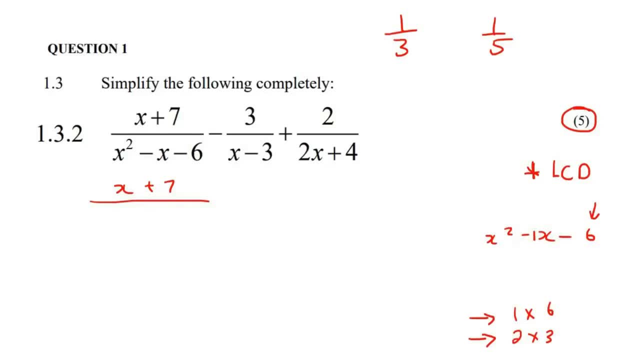 the X And we try to make minus one. So you cannot make minus one using these two numbers, Like six minus one is five. One minus six is negative five. One plus six is seven. You're not going to be able to do it, So it's not that one, So we're going to use these two. How do you make minus one? Well, 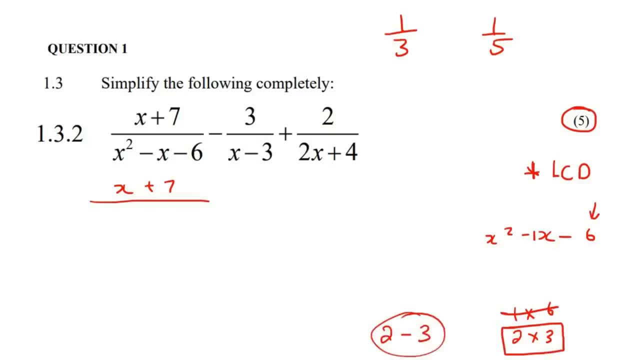 you say two minus three, because that gives you minus one. So we're going to open up two brackets, Okay, And we're going to say X and X, And then we're going to say positive two for this one because it's positive. And then we're going to say positive two for this one because it's positive. 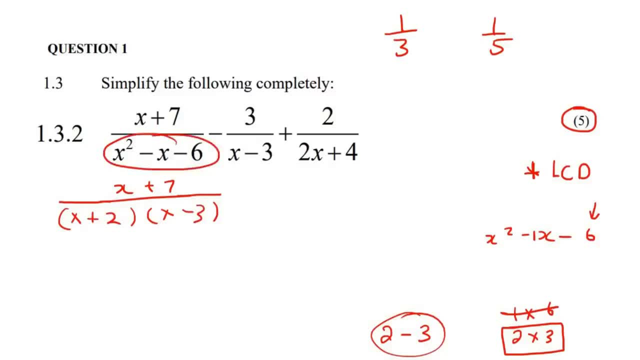 And then negative three, And that is how you factorize that part. Okay, Look at that. X minus three, X minus three- Ooh, something similar. Okay, Now we're just going to leave this part, because this is already factorized. Okay, Now, here you can take out a common factor. 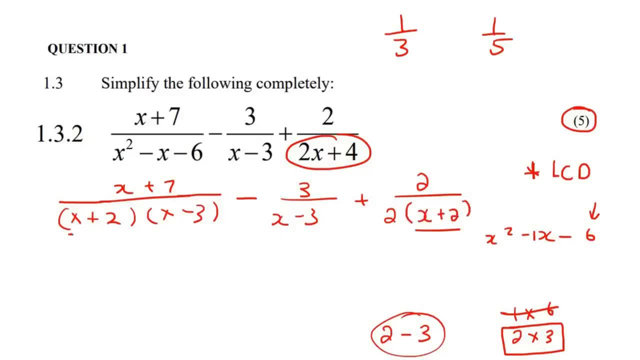 A lot of learners forget about that. And look at that X plus two, X plus two hashtag just saying So you guys must look out for that. Okay, Now to find your lowest common denominator. all you do is you just take all the different parts. 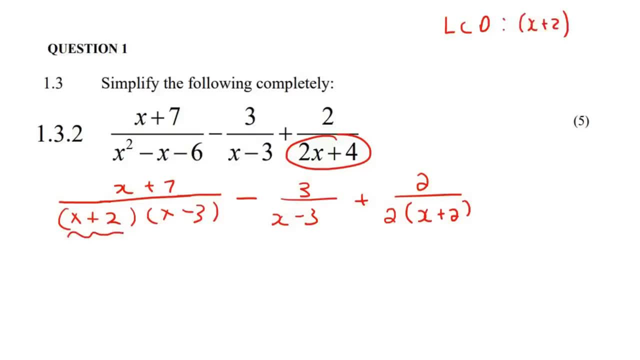 So there's an X plus two- We've got one of those- So that takes care of that and that There's an X minus three. That takes care of that and that. And then there's this random two, which I'll just put in the front, And that takes care of that. Okay, So we've taken care of. 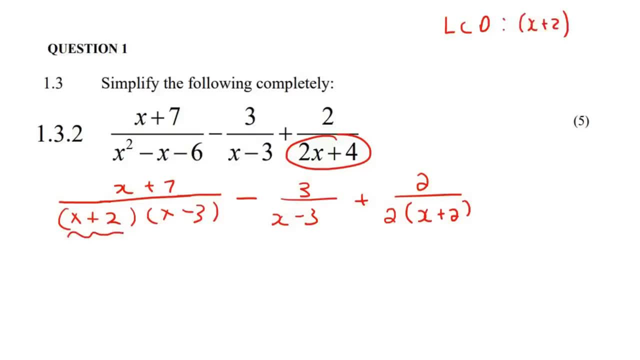 So there's an X plus two- We've got one of those- So that takes care of that and that There's an X minus three. That takes care of that and that. And then there's this random two, which I'll just put in the front, And that takes care of that. Okay, So we've taken care of. 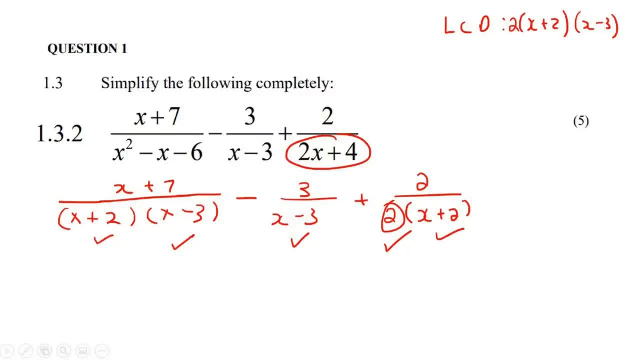 everything. So now what you do? okay, in the next step, you need to make all of these denominators the same as that. So what that means is the following: It means that for this part here, if you look at this part, what is it missing? Well, it's missing the two. So all we'll do is: 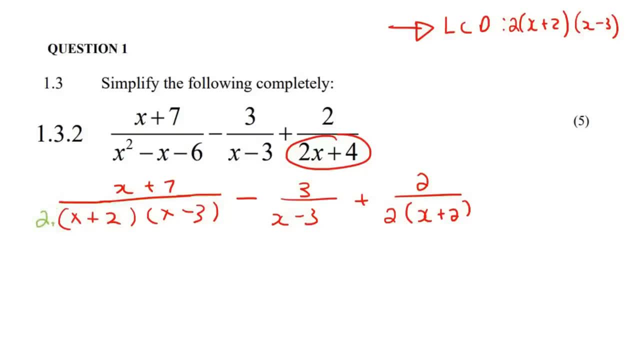 we will put the two there by multiplying. And then what you do to the bottom, you have to do to the top. You see how I put a bracket, Because if I just put a two there, then you would only be giving it to the X. What about the seven? bro? You got to be fair. 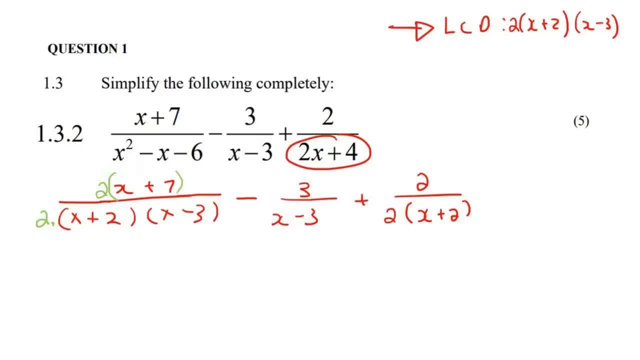 So you got to put it in a bracket so that in the next step we will give it to both. Okay, Excellent. Now we look at this part. Now look at this. What is it missing? Well, it's missing the two, and it's missing an X plus two. So what we'll then do is we'll give it the two and we'll give 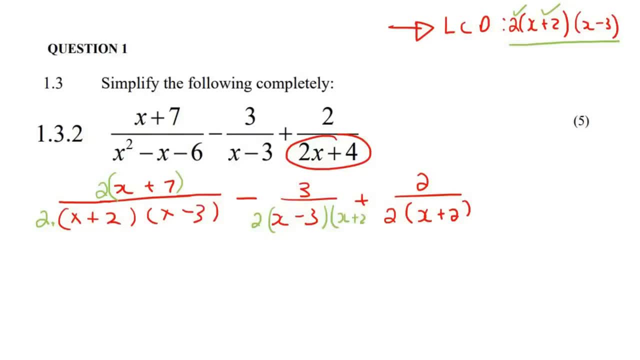 it the X plus two. Okay, See how I used brackets, Because if I didn't, things look really awkward. Like what is that, bro? Come on, You got to do that And you got to do that. Now, what you do to the bottom, you must do to the top. 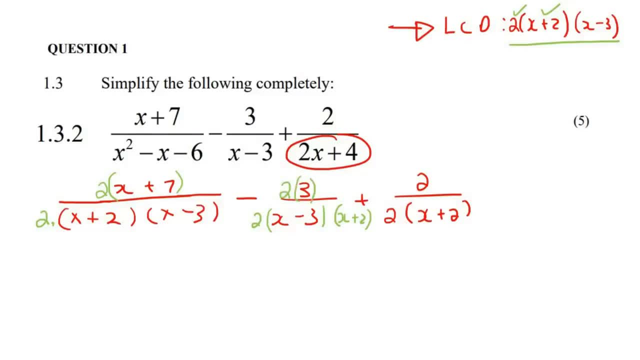 So we're going to give it a two, put a bracket, Otherwise you're going to think it says 23.. And then we're also going to give it the X plus two. Okay, Now we look at this last part. What? 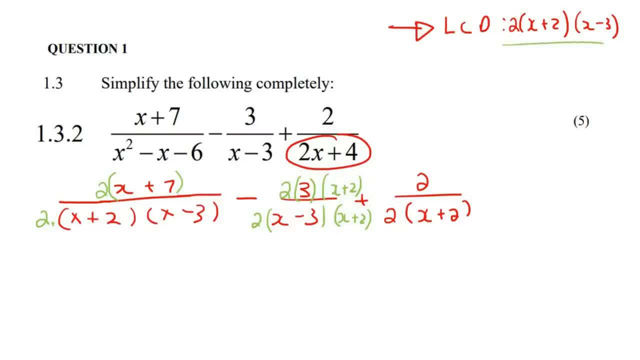 is it missing? If you look at, if you look at this part, well, it's got the two and it's got the X plus two, but it doesn't have the X minus three. So we'll just give it the X minus three. 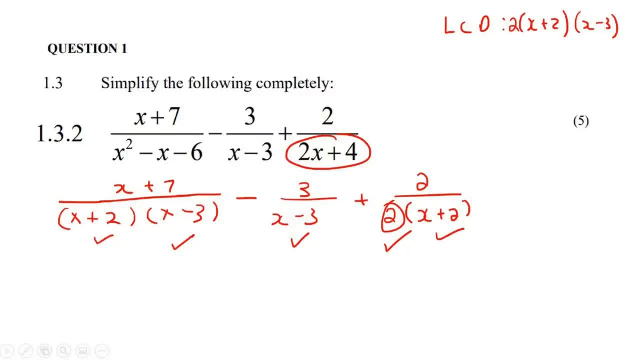 everything. So now what you do? okay, in the next step, you need to make all of these denominators the same as that. So what that means is the following: It means that for this part here, if you look at this part, what is it missing? Well, it's missing the two. So all we'll do is: 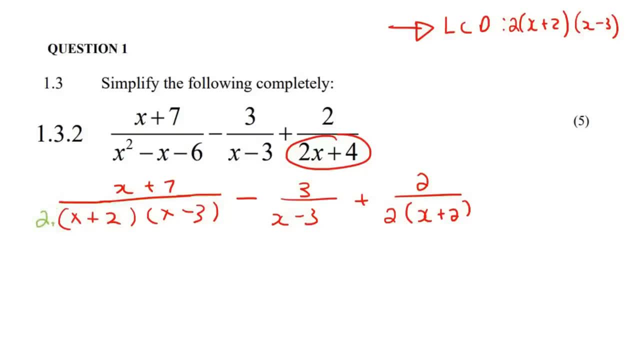 we will put the two there by multiplying. And then what you do to the bottom, you have to do to the top. You see how I put a bracket, Because if I just put a two there, then you would only be giving it to the X. What about the seven? bro? You got to be fair. 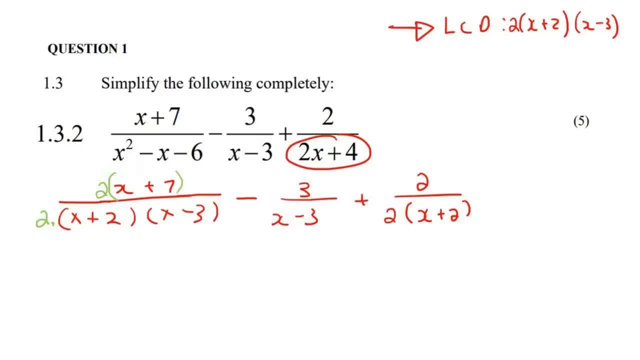 So you got to put it in a bracket so that in the next step we will give it to both. Okay, Excellent. Now we look at this part. Now look at this. What is it missing? Well, it's missing the two, and it's missing an X plus two. So what we'll then do is we'll give it the two and we'll give 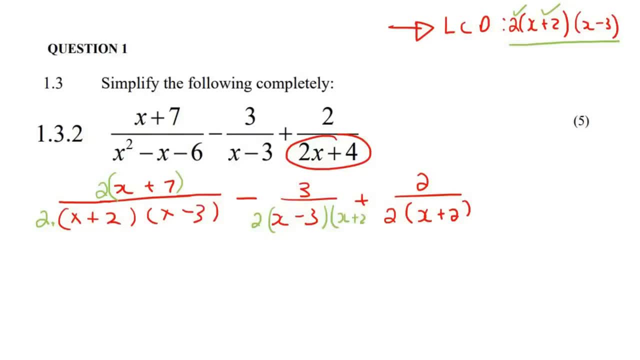 it the X plus two. Okay, See how I used brackets, Because if I didn't, things look really awkward. Like what is that, bro? Come on, You got to do that And you got to do that. Now, what you do to the bottom, you must do to the top. 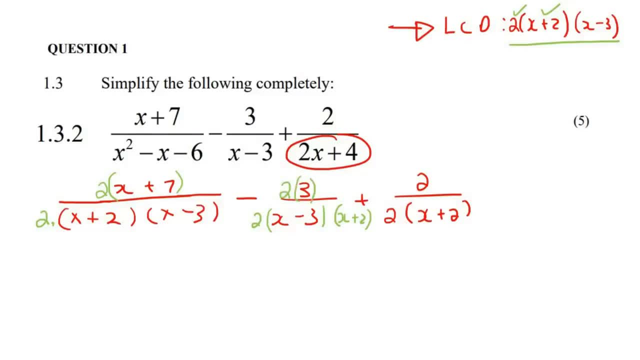 So we're going to give it a two, put a bracket, Otherwise you're going to think it says 23.. And then we're also going to give it the X plus two. Okay, Now we look at this last part. What? 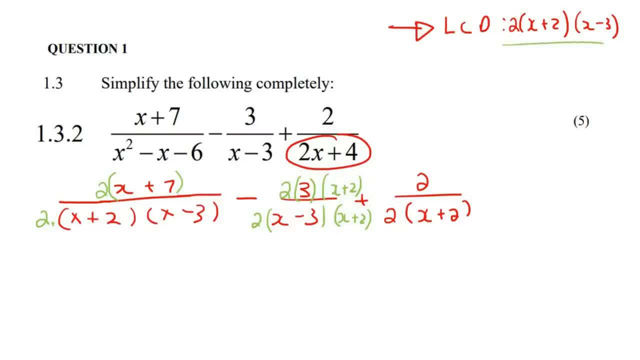 is it missing? If you look at, if you look at this part, well, it's got the two and it's got the X plus two, but it doesn't have the X minus three. So we'll just give it the X minus three. 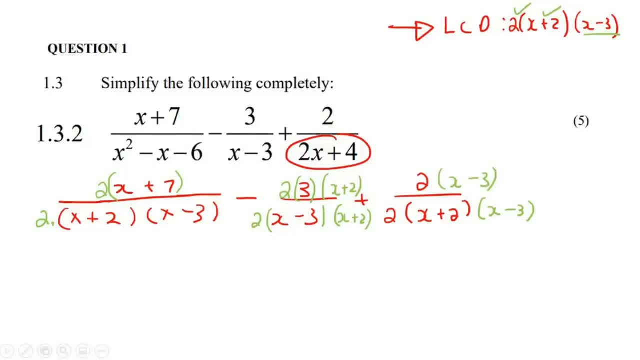 What you do to the bottom, you do to the top, And there we go. Now what we are going to do is we're just going to put one long line, Okay, And you're going to put the bottom part like that, but we're not going to multiply the bottom part out. It's weird. 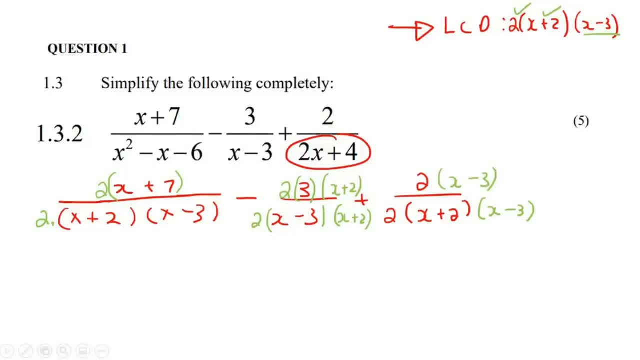 What you do to the bottom, you do to the top, And there we go. Now what we are going to do is we're just going to put one long line, Okay, And you're going to put the bottom part like that, but we're not going to multiply the bottom part out. It's weird. 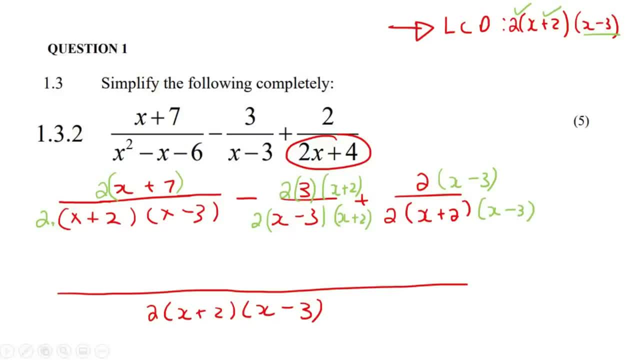 right. I know that when you simplify you're supposed to get rid of brackets, but not in the denominator. For some reason we we um. as mathematicians they love to keep the denominator in the um factorized form, like that. But at the top I just want you to go write everything out Now. 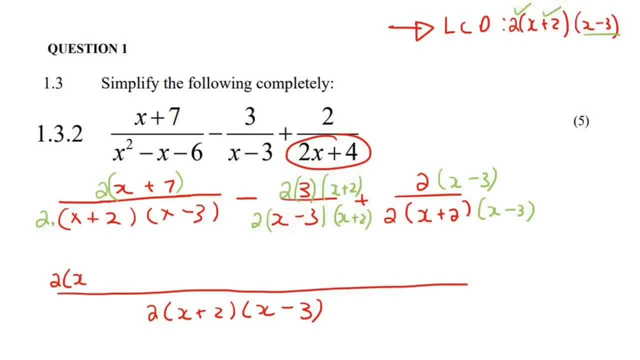 please don't multiply anything together yet. Um, it's going to cause some issues, Trust me. So then what you do is you just say minus, and then you just say two times, three times, X plus two, And you just say plus. there we go. Now at the top. we have some work to do, We have to go. 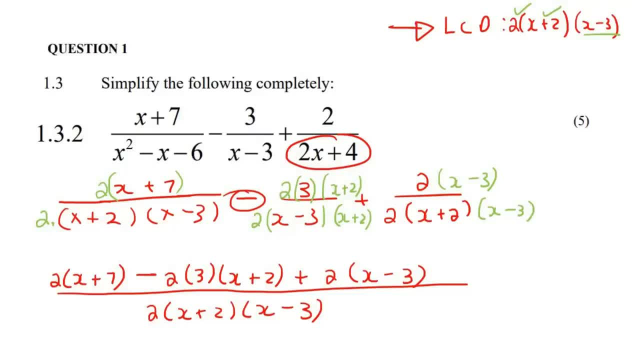 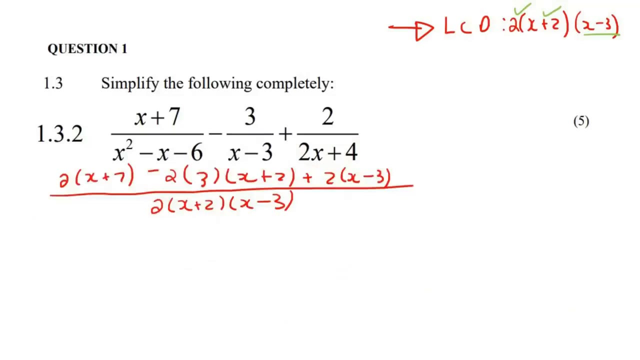 get rid of all the brackets at the top, Okay. So at the bottom we just keep it as it is. Okay, I hope I have space. So you're going to multiply this two into this bracket, So that's going to become two X plus 14.. All right, My apologies, I had to go make a bit of space, So 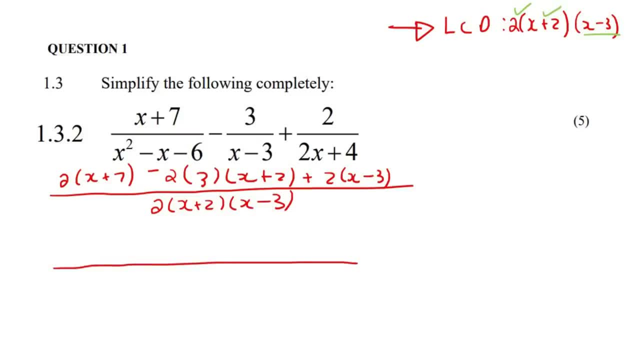 I erased the one step, Um, and now I've got this. Okay, So that means we have two, X plus two and X minus three. Okay, So, as I said, we're going to multiply the two into that bracket, So you become: 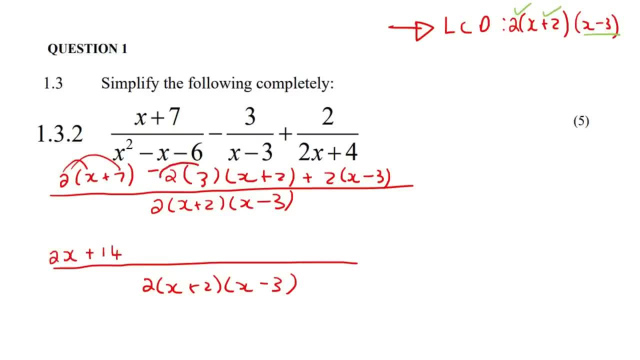 two X plus 14.. Now here, just put these two together, So that'll just be negative six, And then X plus two, And then multiply this out So that'll become two X minus six. Let's quickly do the step over here. 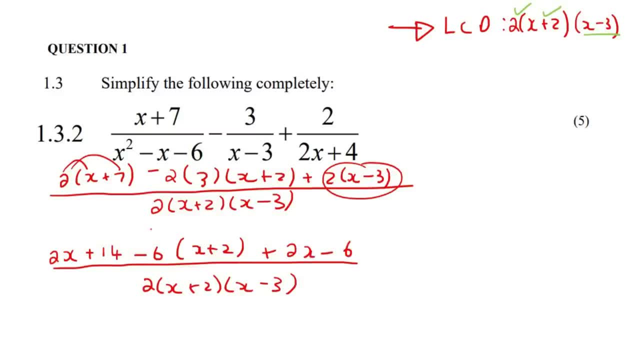 So, uh, minus six times X is going to be negative six X, And then minus six times positive two is going to be minus 12.. So, minus six X minus 12, minus six, minus six X, minus 12.. And there we go. 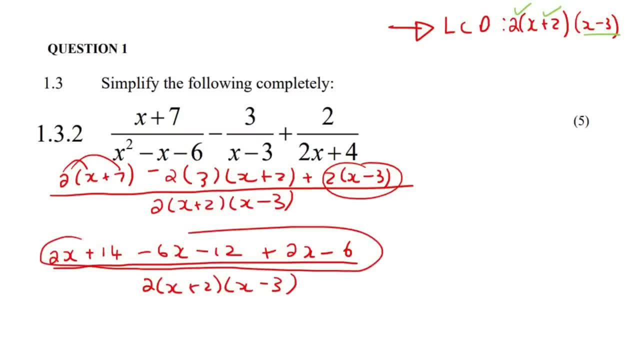 Okay, Now at the top you're just going to put all the like terms together. So you've got an X, another one, So that's two minus six plus two. So two minus six is minus four. minus four plus two is minus two. 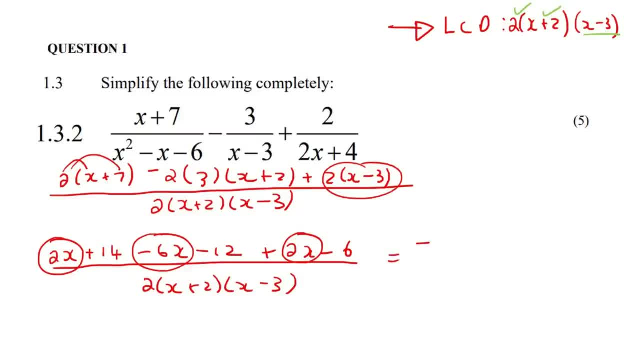 Okay, Uh, let's actually just write the answer here. What did we say to minus two? Okay? And then we have 14 minus 12, which is two, and then two minus six is minus four. And then at the bottom here, you are going to do this, Okay. 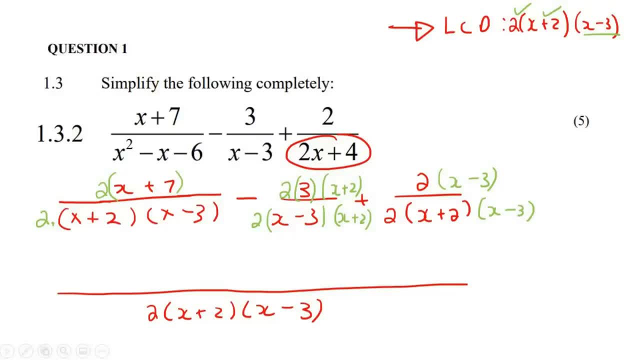 right. I know that when you simplify you're supposed to get rid of brackets, but not in the denominator. For some reason we we um. as mathematicians they love to keep the denominator in the um factorized form, like that. But at the top I just want you to go write everything out Now. 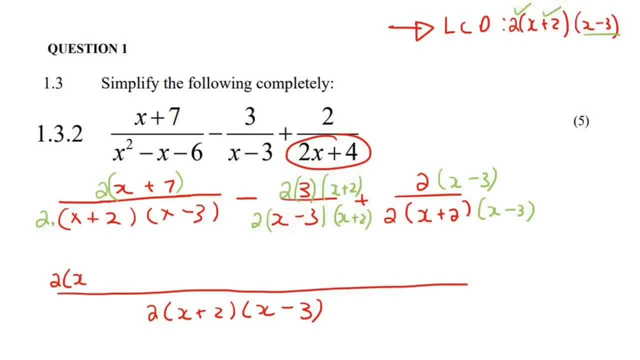 please don't multiply anything together yet. Um, it's going to cause some issues, Trust me. So then what you do is you just say minus, and then you just say two times, three times, X plus two, And you just say plus. there we go. Now at the top. we have some work to do, We have to go. 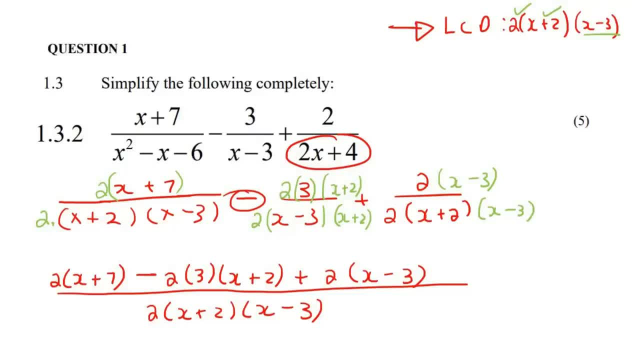 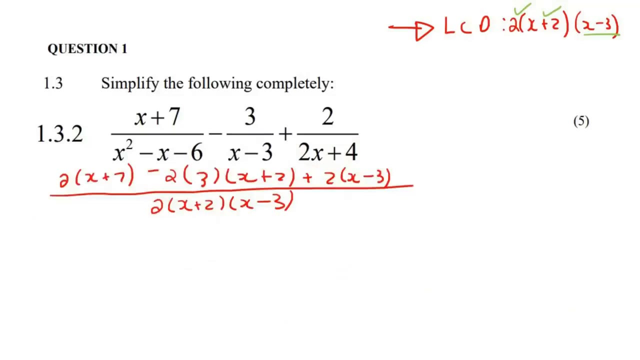 get rid of all the brackets at the top, Okay. So at the bottom we just keep it as it is. Okay, I hope I have space. So you're going to multiply this two into this bracket, So that's going to become two X plus 14.. All right, My apologies, I had to go make a bit of space, So 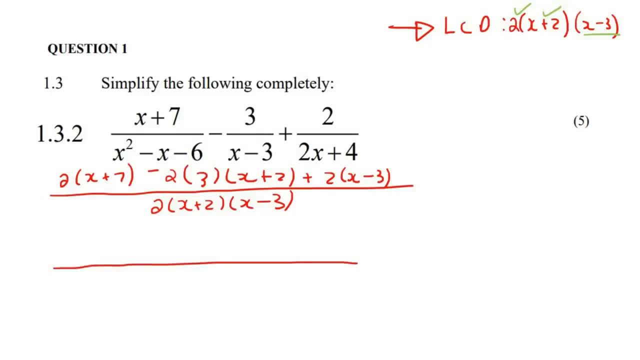 I erased the one step, Um, and I've got this. Okay, So that means we have two X plus two and X minus three. Okay, So, as I said, we're going to multiply the two into that bracket, So you become two X plus 14.. Now here, just put these two together, So that'll just be negative six. 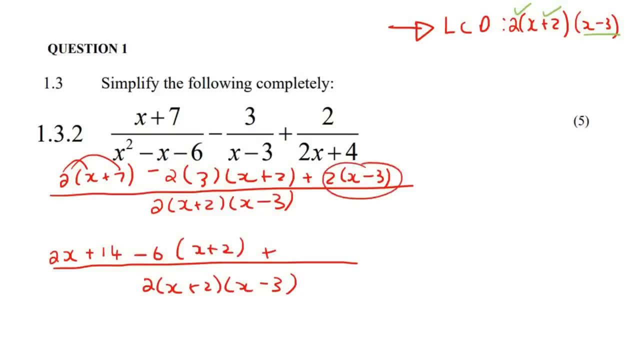 and then X plus two, two and then multiply this out so that'll become two x minus six. let's quickly do the step over here. so minus six times x is going to be negative six x, and then minus six times positive two is going to be minus twelve. so minus six x minus twelve minus six, we'll give minus six x minus. twelve. and there we go. okay, now at the top you're just going to put all the like terms together. so you've got a x, another one, so that's two minus six plus two. so two minus six is minus four, minus four plus two is minus two. okay, let's actually just write the answer here. what did we say? two, 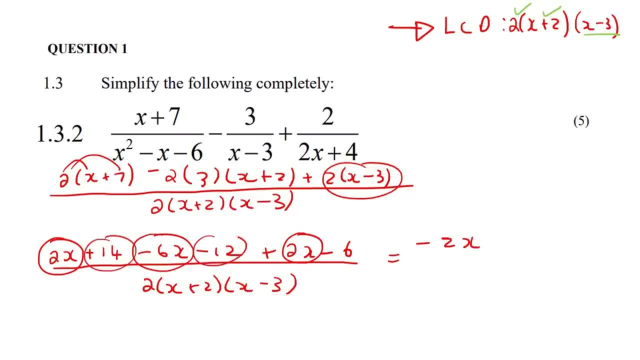 yeah, minus two, okay, and then we have fourteen minus twelve, which is two, and then two minus six is minus four. and then at the bottom here you are going to do this. okay, now you just need to do another little check at the top to make sure we can maybe. 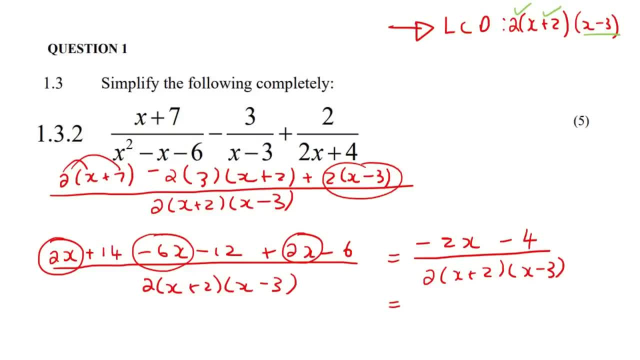 factorize further- and in fact we can. we can take out a negative two, and then you'd be left with x plus two. how do I do that? we'll check here. if you multiply these two together, what do you get? negative two, x. and if you multiply these two together, you get negative four, which is what 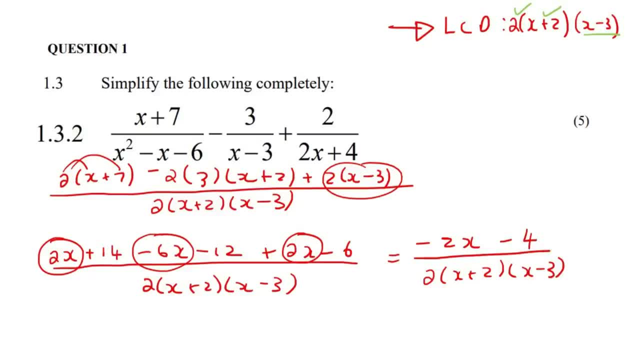 So we just need to do another little check at the top to make sure we can maybe factorize further, And in fact we can. we can take out a negative two, and then you'd be left with X plus two. How do I do that? We'll check here. If you multiply these two together, what do you get? 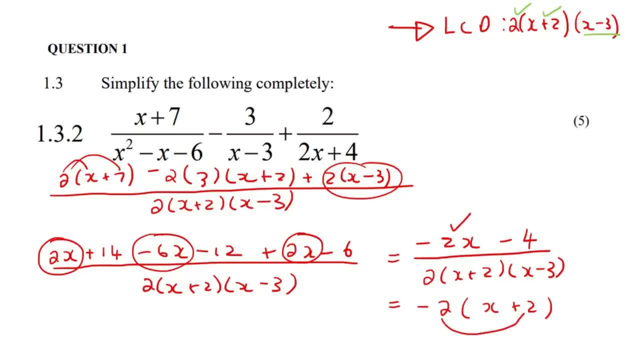 Negative two, X, And if you multiply these two together you get negative four, which is what we had Now. the reason I did that is because if you now look at the bottom, we have things that can. that can cancel out Okay. 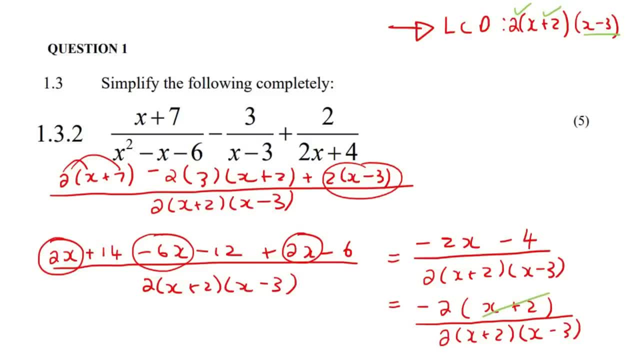 So here we're going to have those cancel out, and the twos can also cancel out, And so for our final answer, you're going to have minus one at the top, because there's nothing there except the little negative, And then at the bottom 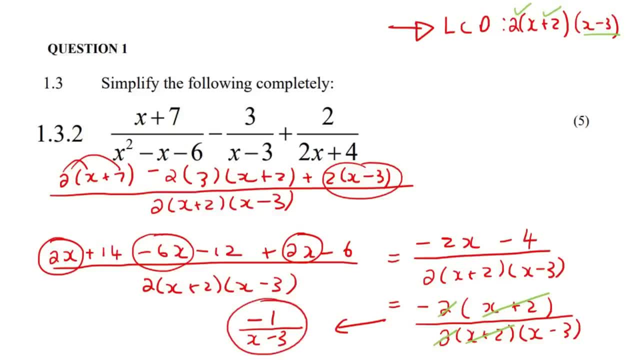 you're going to be left with X minus three, And that is our final answer. 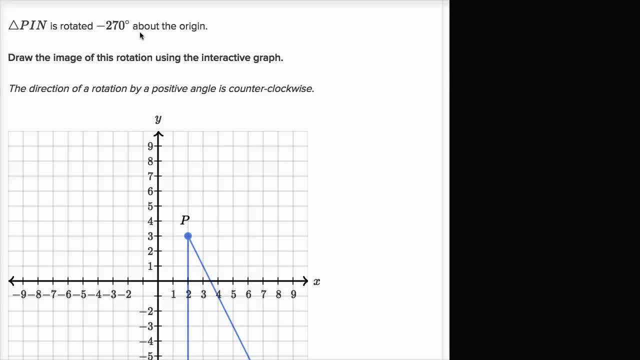 We're told that triangle PIN is rotated negative 270 degrees about the origin. So this is the triangle PIN. We're gonna rotate it negative 270 degrees about the origin. Draw the image of this rotation using the interactive graph: The direction of rotation by a positive angle. 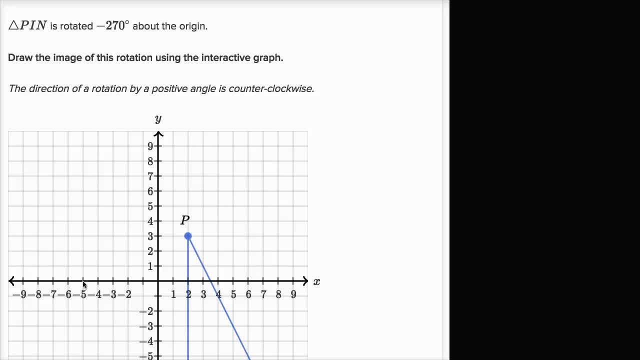 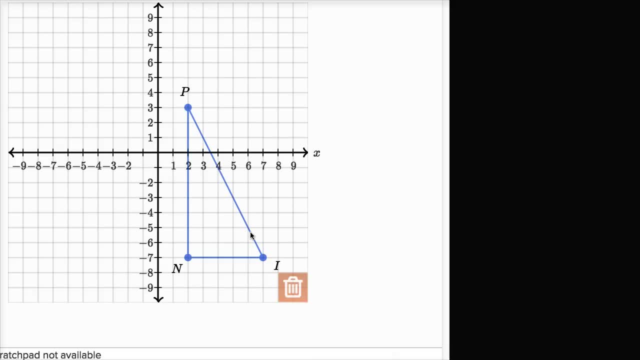 is counterclockwise, So positive is counterclockwise, which is the standard convention, And this is negative, so negative degree would be clockwise And we wanna use this tool here And this tool, I can put points in or I could delete points. 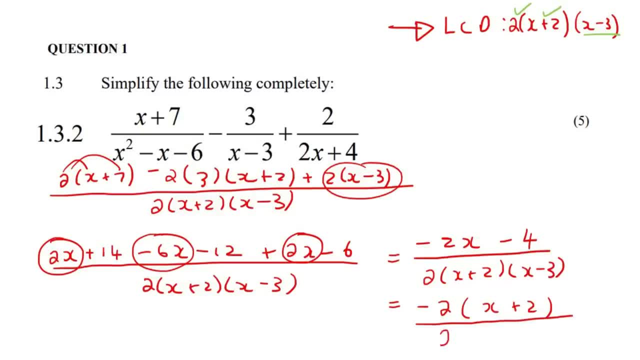 we had now. the reason I did that is because if you now look at the bottom, we have things that can, that can cancel out. so here we're going to have those cancel out, and the twos can also cancel out, and so for our final answer, you're going to have minus. 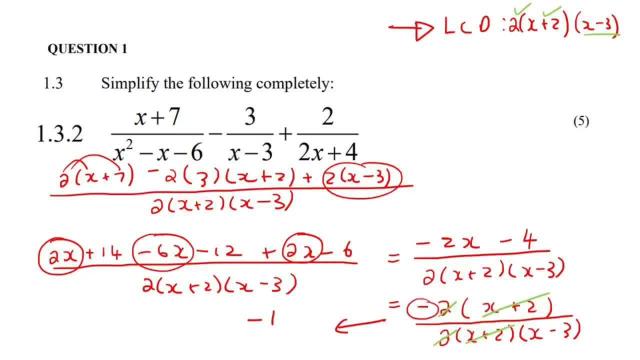 one at the top, because there's nothing there except the little negative, and then at the bottom you're going to be left with x minus three, and that is our final answer. 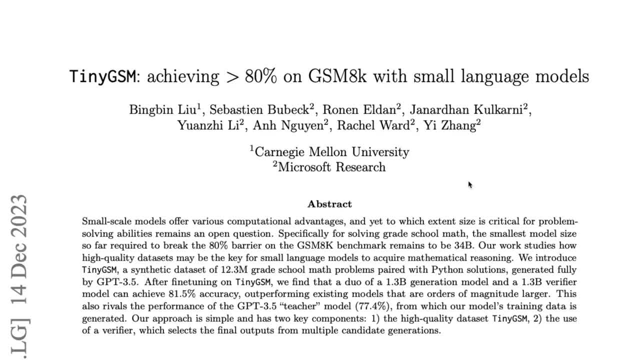 Either we have a terrible understanding of what happens inside a large language model, which is partly true, or our obsessive nature to go after benchmarks are going to hurt us in the 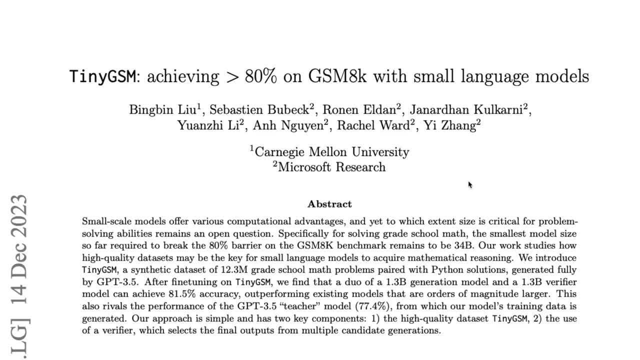 long term. But either way, there is a new paper. This is definitely not a rant. I don't want to have this video as a rant, but I have some strong opinions about this particular paper and what I feel is a problem in pursuit of benchmarks. First of all, this paper is called Tiny GSM. 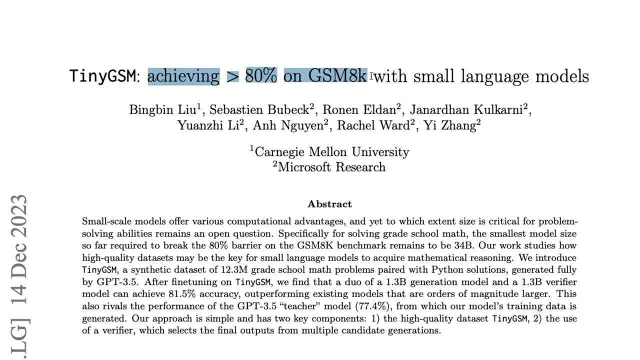 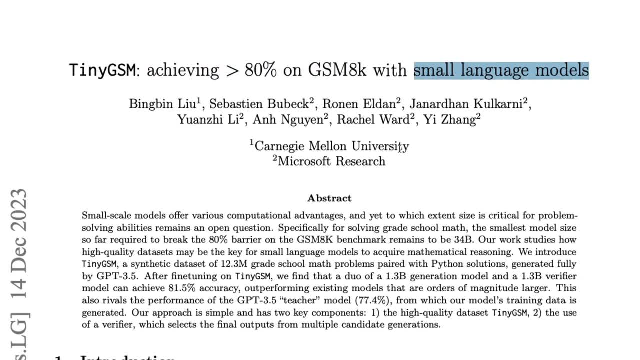 The paper says it is achieving greater than 80% on GSM 8K, which is a benchmark dataset with small language models. I know Microsoft is obsessed with this word called SLM, and I saw Satya Nadala talking a couple of times about SLM on different occasions, and they recently released PHY model, which I've still not yet covered. So Microsoft is obsessed with this word or the term called SLM. 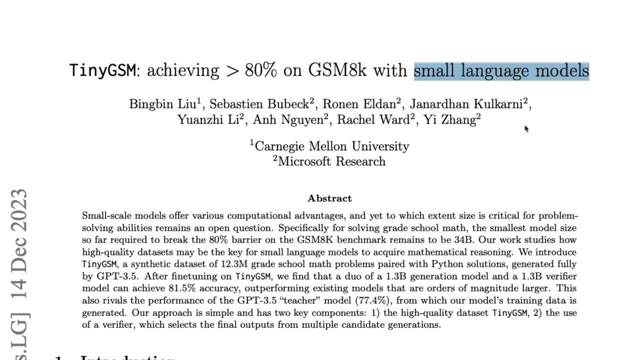 I don't know, for some reason they want to call it SLM, not like small, large language model, but they want to call it SLM, not like small, large language model, but they want to call it SLM, not like small, large language model, but they want to call it SLM, not like small, large language model, maybe they found it oxymoron-ish. But this is a paper from Carnegie Mellon University and Microsoft